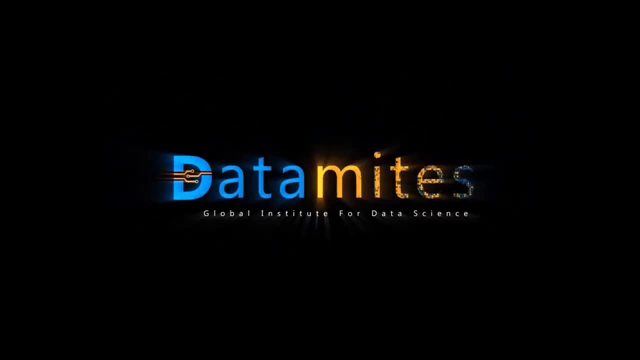 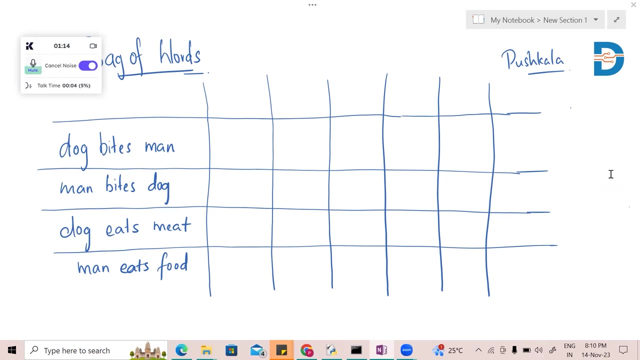 Hello learners. this is Pushkala and we are going to see what is bag of words in text processing. So let's first start. So we'll be going on with a few sentences. So let's assume this is my sentence 1, 2,, 3 and 4.. So let's say how bag of words work. Let's say you're working with a. 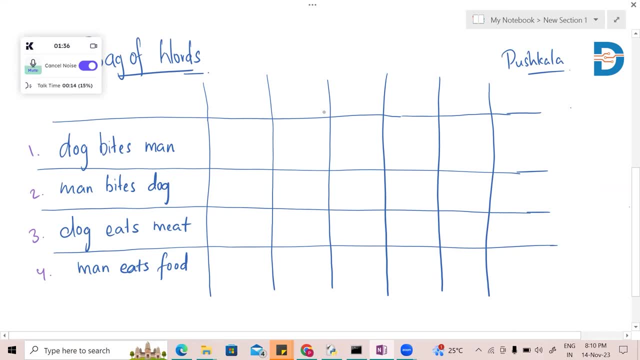 text data set. Text data set is not as easy as numerical data set. While going for text classification and everything, you cannot directly process text in some algorithms. So in that case you will have to convert this text into numerical form. So to convert this text, 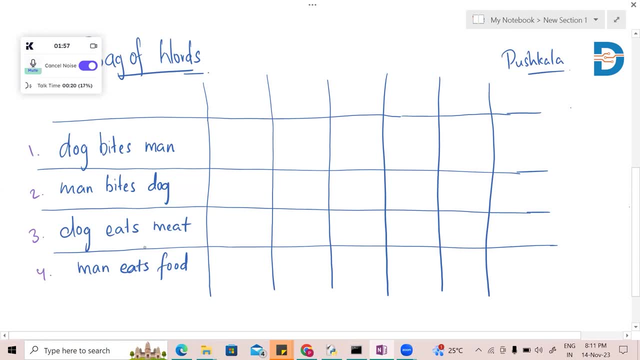 data to convert this text into features, that is, numerical features. how can we do that is? we'll find out here. So each of the unique words in this sentence, So each of the unique words is dog bites man, and there is no unique words here and here it's eats and meat. 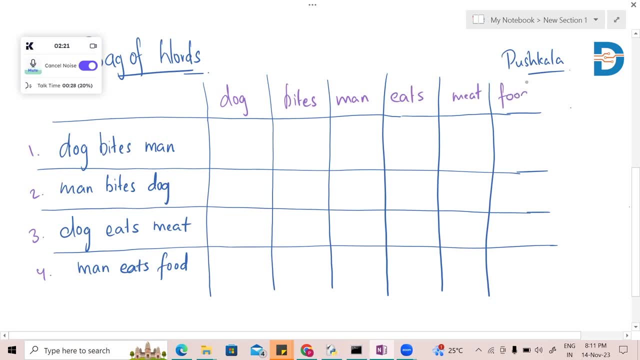 And in the last sentence, I have food as the unique word. We have these many unique words in these four sentences, And what we will be- how we will be converting this particular sentence into a numerical data- is: these are my independent features. 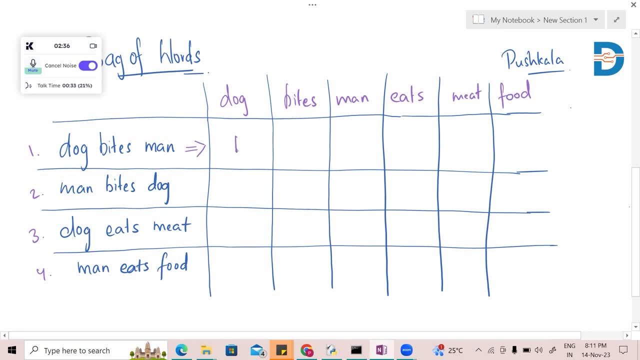 Now from this I'm going to say: dog, I have the occurrence of one time Bites, one time Man, one time, And all of these words is not present in this particular data, So I'll be giving the count here. 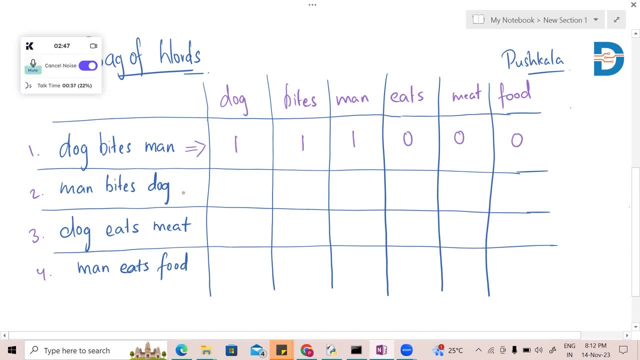 So man bites dog 1,, 1.2.. And all of the other: 0.7,, 1,, 1,, 11, and 0, 01, and it doesn't have zero. All I'm going to create it on my own. 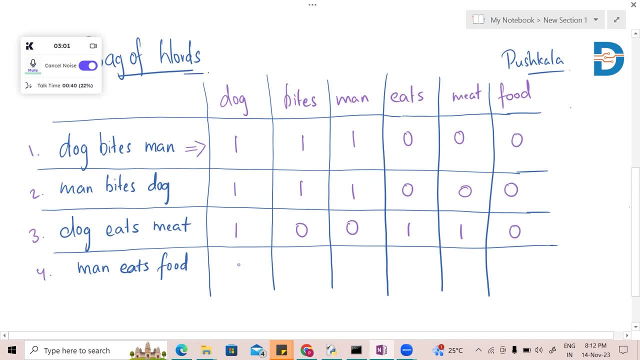 So what I can do is let me limit my tableart to zero Right now. So let's say What? 01.. 30., 30., 31.. have dog or bites? it has man eats. meat is 0 and food is 1.. So this is how we convert. 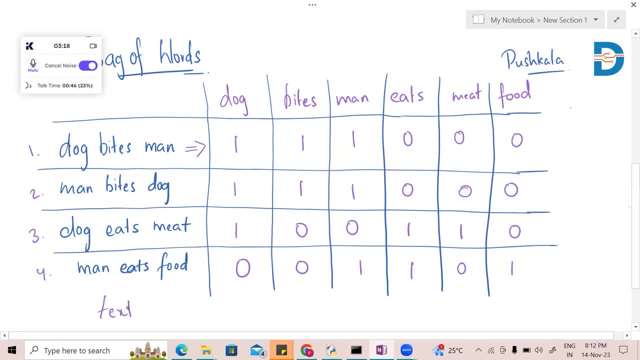 this text into numerical features. So for the algorithms that doesn't support text directly, you can convert this into a numerical feature and feed it into the computer. So that is how it does. So let's say, I have dog here one more time, so this feature will be turned. 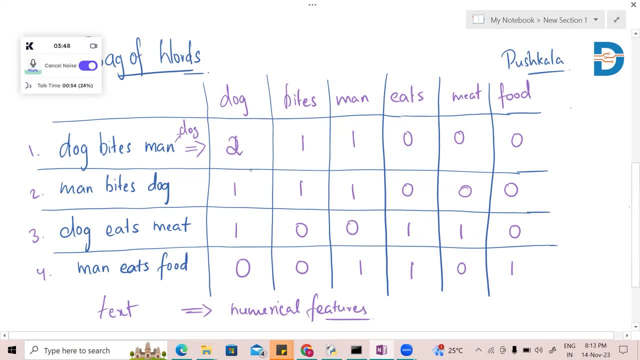 out to be food. That is how bag of words works. It will write down the number of count. the particular word occurs that sentence. So this is bag of words and for a Python implementation to implement this bag of words, we have some function called foundVectorizer. We will be using this foundVectorizer. 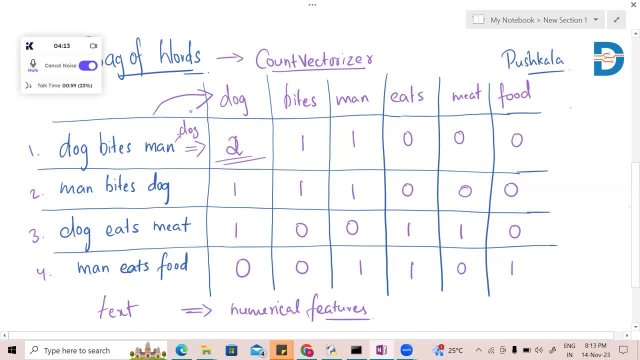 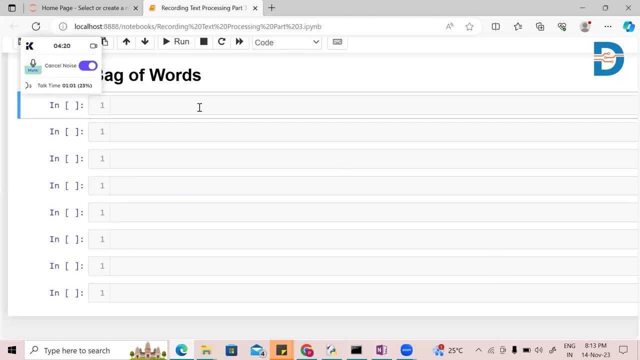 function to convert the sentences into a numerical feature. So let's start. I will be going into the Jupyter Notebook and let's import the necessary libraries. So I will have only one. I need only one library from feature extends txt. import foundVectorizer again and then 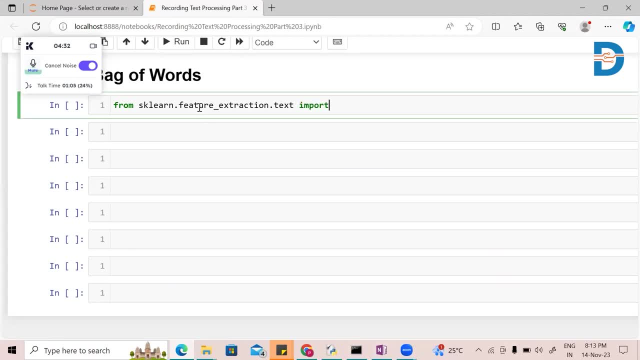 vote. This is the library I need them From scale on feature extraction and that's importing foundVectorizer. So let's say we have this document Txt and I am- I'll be writing all of the text inside: dog bites and bites dog. 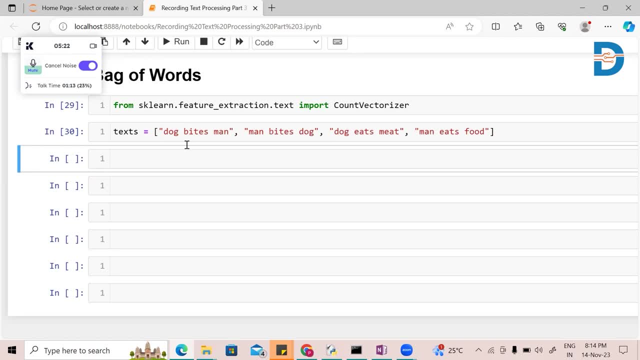 So I have done that, So we have all the four sentences here and we don't have any special characters or punctuations or uppercases to remove. I have specifically done the text like that. If not, you will have to go through some pre-processing steps before going into the count vectorizer. 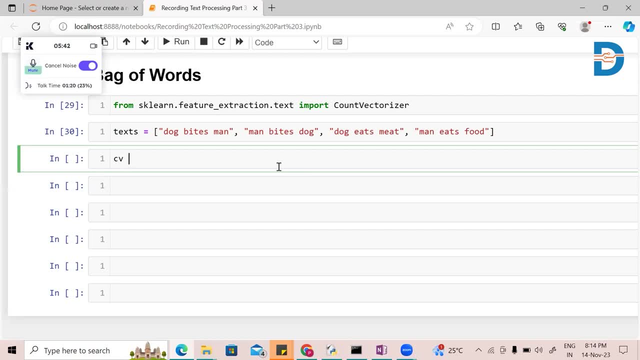 So let's start. Let's say count vectorizer is C. Okay, So count, So count vectorizer. what I'm going to use is: I'm going to call this function, So count vectorizer is called. Now I'm going to use bag of words. 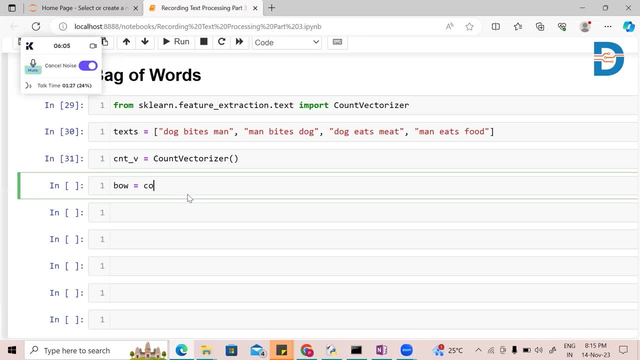 In this bag of words. I'm going to use this count vectorizer function And inside that I'm going to say fit and transform. This is practically a pre-processing step, So I'm asking the system to learn That is fit. 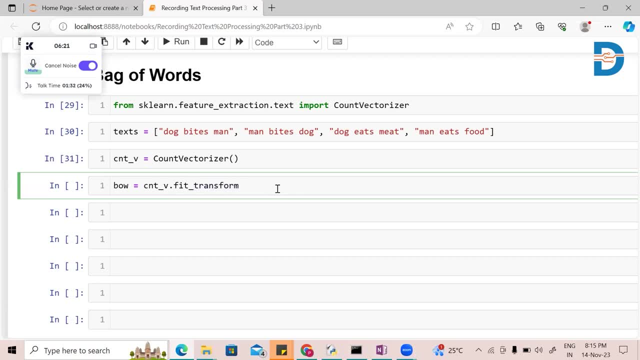 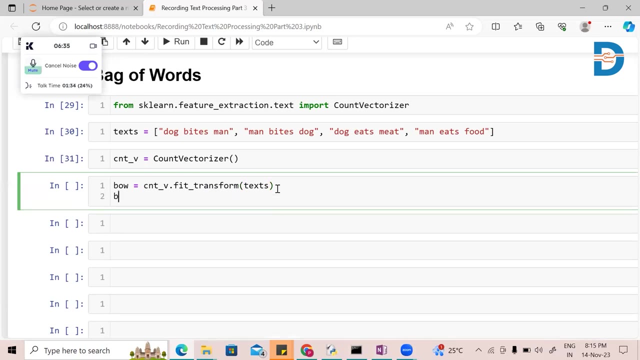 Asking the system To learn And then transform it into a numerical function. So this is what fit and transform function does, And I'm going to use it's tensile And when I print it, see what happens. Okay, Yeah. 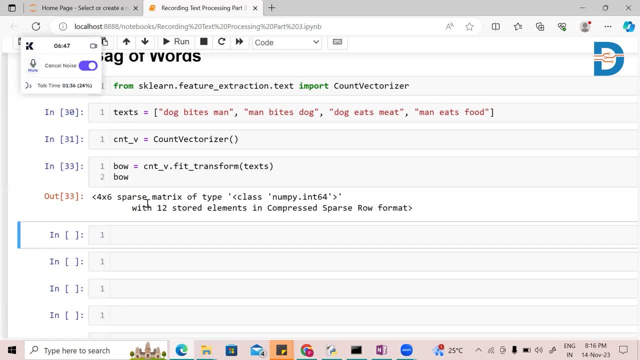 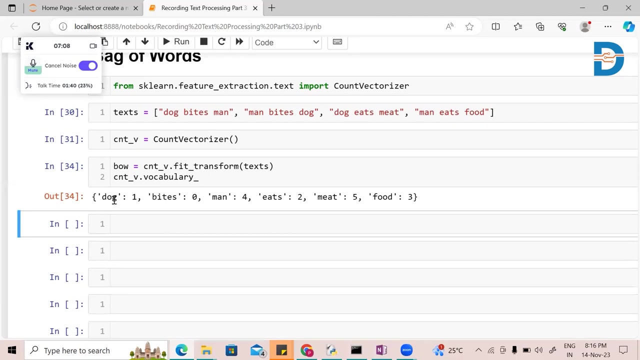 So it doesn't print anything much. It does it though. So what we are going to do is I'm going to call A function called vocabulary. That has to be done with the count vectorizer Vocabulary function. I have about six features: dog bites, man eat. this is what we have seen in this representation as well. 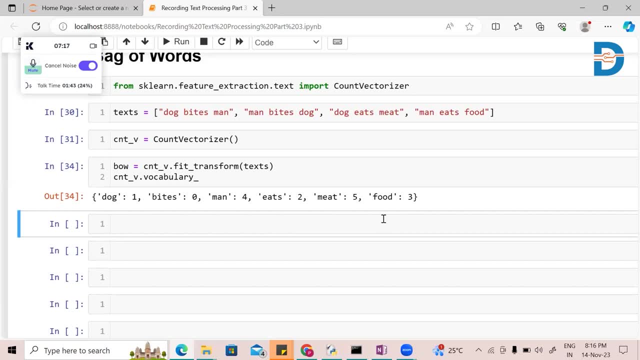 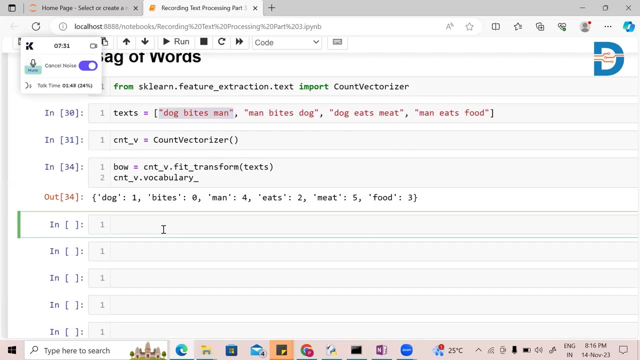 So we have about six features and let's see the how the bag. Okay, So for the first sentence: dog bites man. what is the bag of words representation for this? I can use this and zero. It doesn't do much. 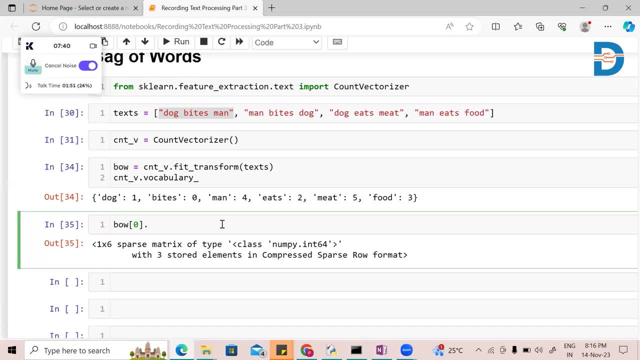 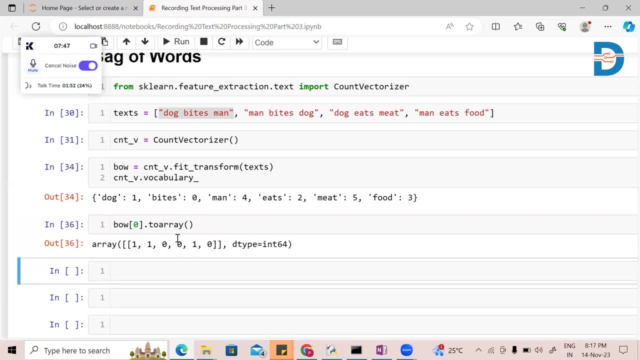 So I'm going to convert this into our. it is displaying object. Object cannot be viewed, So I'm going to transform this into a array. That's it. This is for the first word, Where I know bites goes first. bites is the first feature, dog is the second feature. 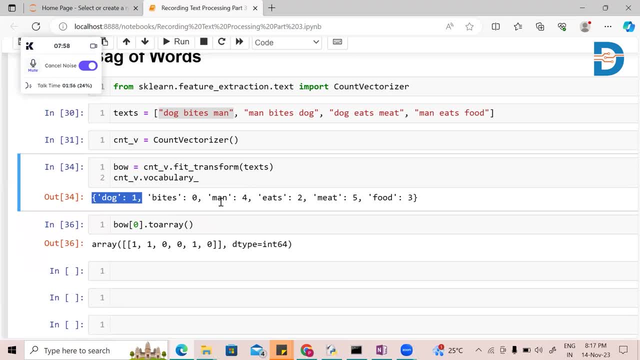 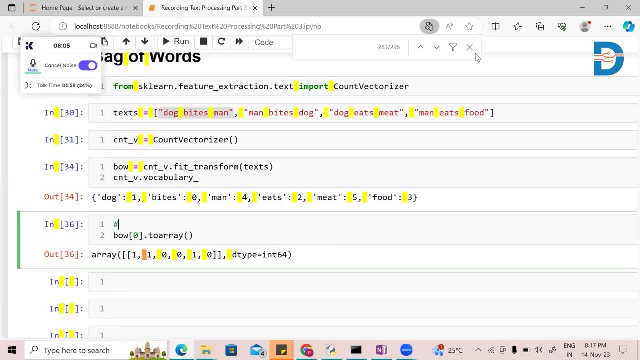 So go with the zero: one, two, three, four, five. So let me write that representation So it's going to be easy for you guys to. The first feature is bites- They can feature this dog, dog. And third feature is eats and food, man. and this is my features and the first sentence contains bites, dog and eats, and food is zero and man is one.